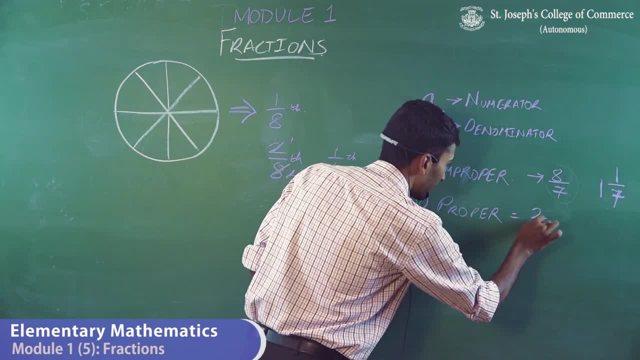 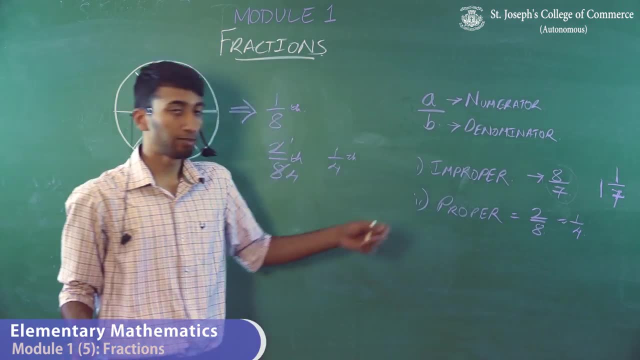 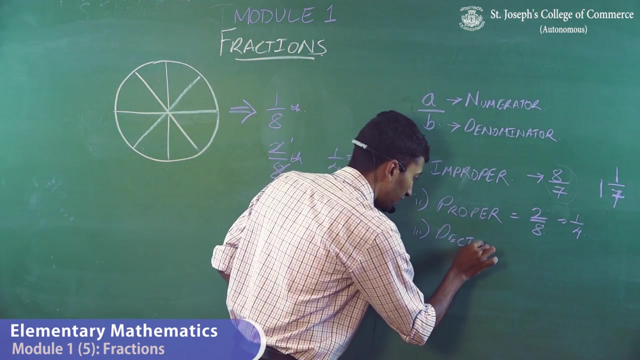 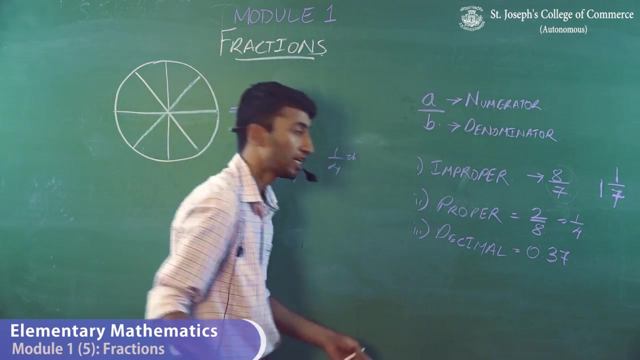 is actually something like 2 by 8, as given in the example. So 2 by 8 can be written as 1 by 4.. That is proper. And then there's something called as decimal fraction Where, say, for example, 0.37 is your decimal. To convert that into a fraction: 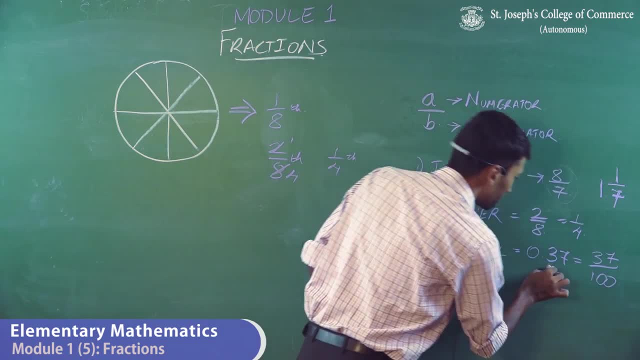 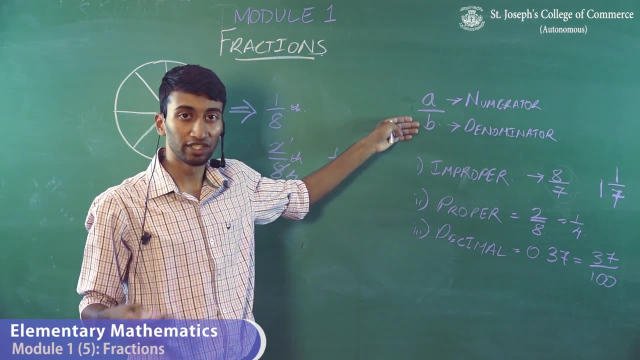 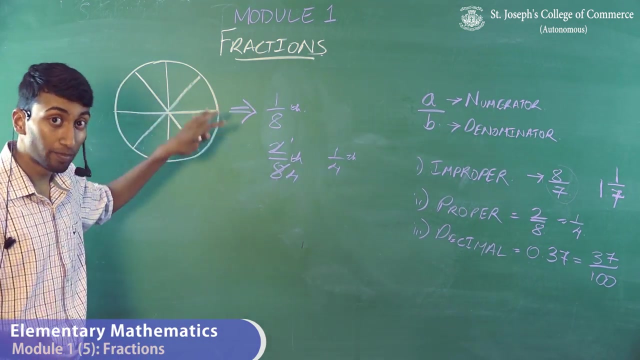 it is 37 by 100.. So 0.37 is your decimal fraction. So now B is greater than B. So B generally does not equate to 0.. As say, for example: out of 8 parts you've eaten. 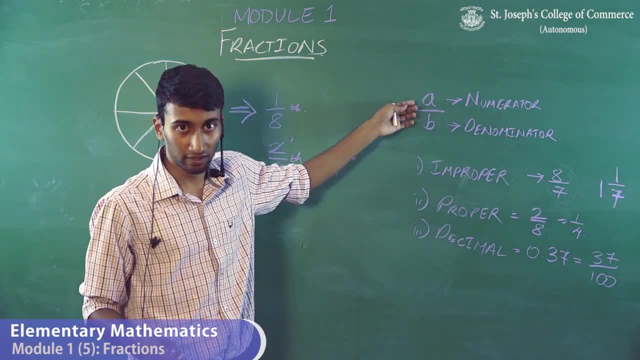 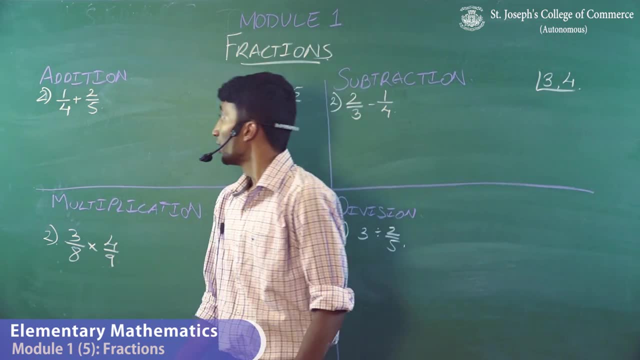 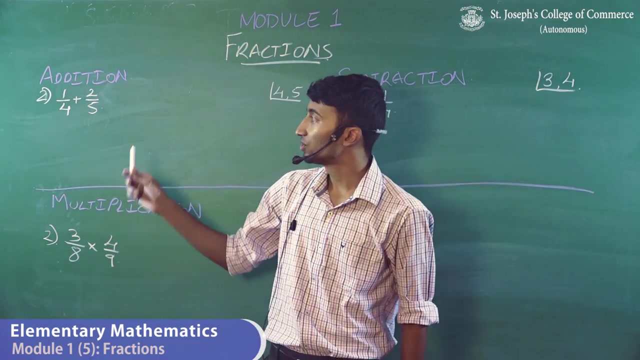 one part Now out of 0 parts. you can't eat anything, So that is why B is generally not equal to 0.. So now we'll move into solving fractions. So there are four different things: Addition, subtraction, multiplication and division, wherein we will solve one sum under. 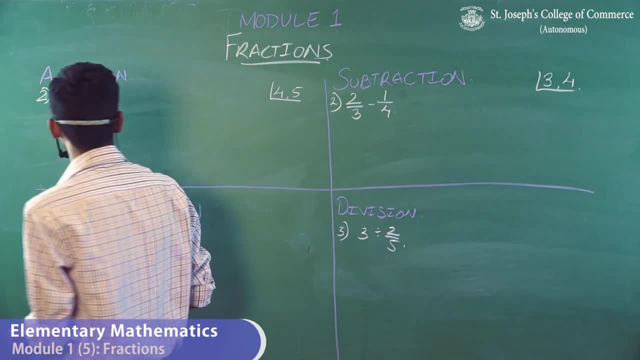 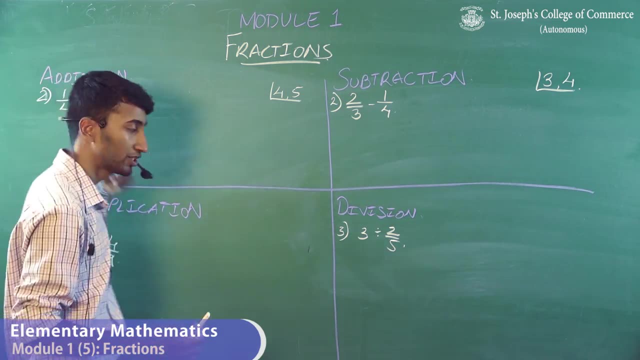 each of these. So, when it comes to addition of fractions, so I'm taking the second sum under addition, that is, 1 by 4 plus 2 by 5.. So now, as you know, as you can notice, the denominators: 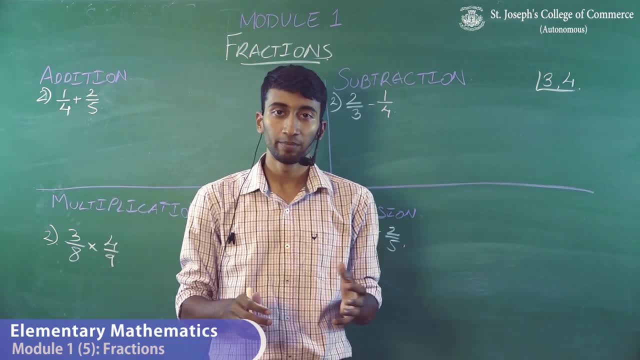 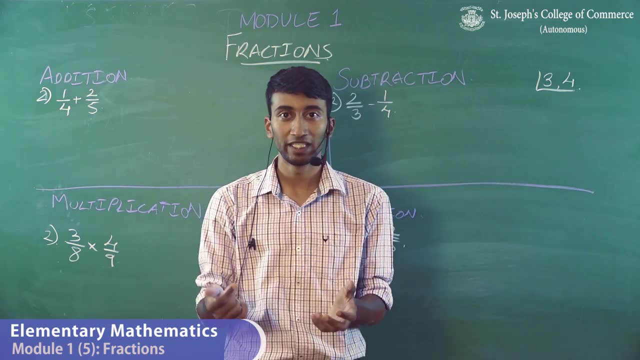 are not the same. That means you cannot add a pizza which is 4 parts and a pizza which is 5 parts. Their sizes will be different. So what you have to do is you have to take the LCM of these two numbers. 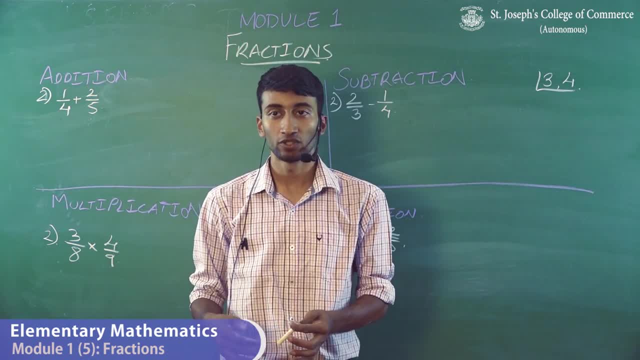 So all you have to do is take the L-C-M of all pairs So that you get the denominator equal. Then you solve it. So you take the LCM of 4 and 5.. So 2 plus 2 is 4.. 2, 5 is 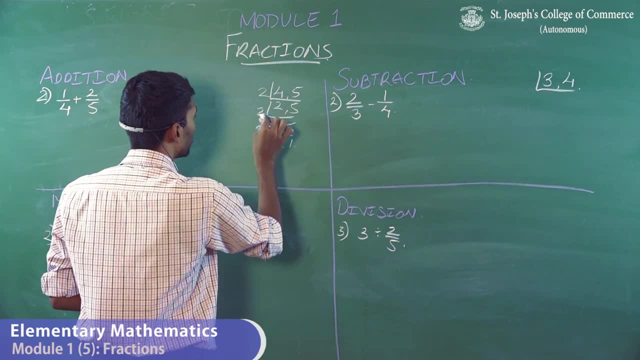 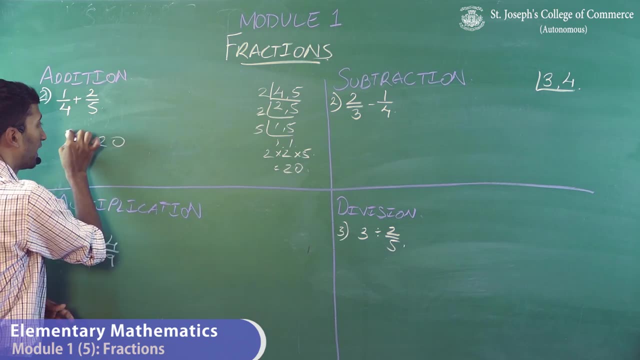 5.. 2 times 2, 1, so 2 is 1.. 5 times 2, 1 is 5.. So 2 plus 2, the derivative of 5, that gives you 20.. So now, 20 is your LCM. 4 equales 5 is equal to 20.. So now, since 4 makes 4 equal, 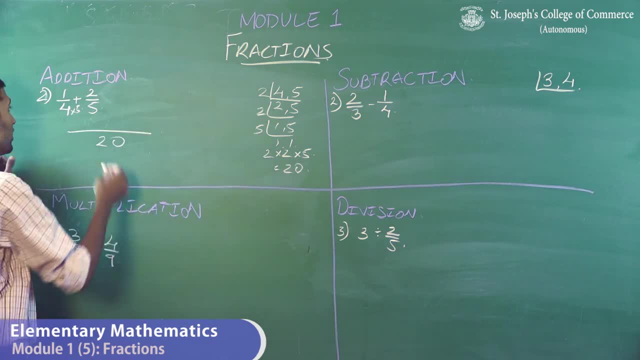 to 5, so 4 x 5 equals 20.. If you are multiplying the denominator by 5,, you should multiply the numerator also by 5.. So you multiply 1 into 5, that you will get 5, plus, and 5, 4s are 20, 5 into 4 will give. 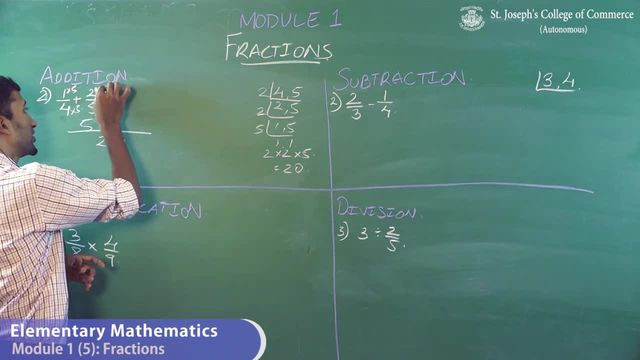 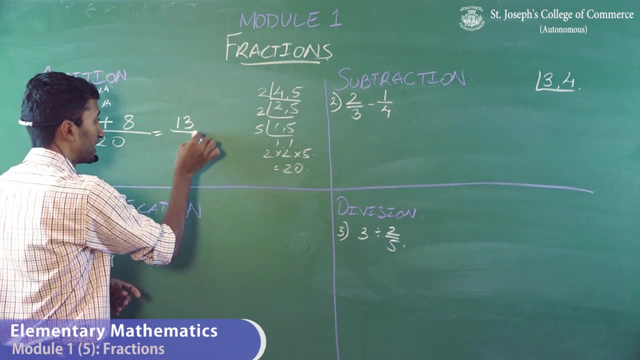 you 20.. So if you are multiplying the denominator by 4, you multiply the numerator also by 4.. So 4, 2s are 8.. So 5 plus 8 will give you 13, by 20.. So this is how you add. 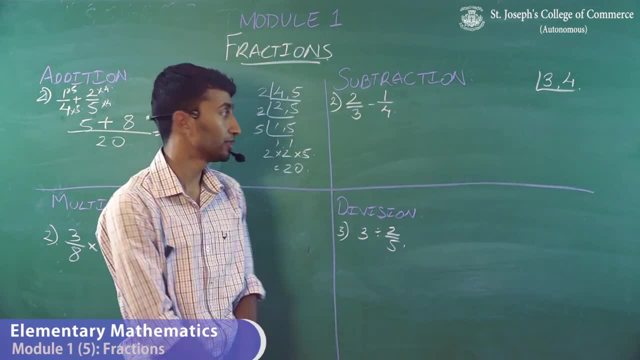 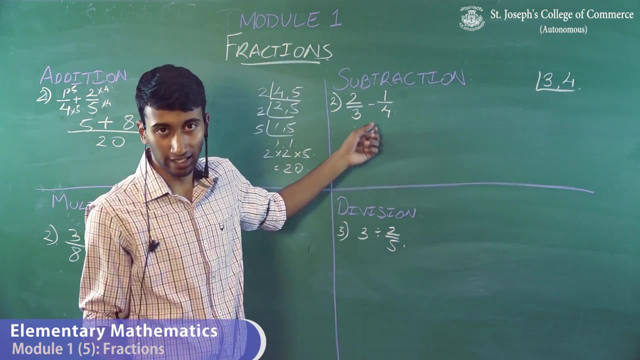 So we move into subtraction, where we solve the second sum. under subtraction, that is 2 by 3 minus 1 by 4.. As you can notice, the denominators are not the same, so you have to take the LCM. 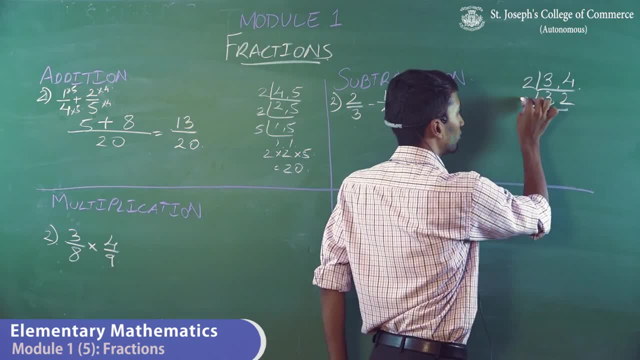 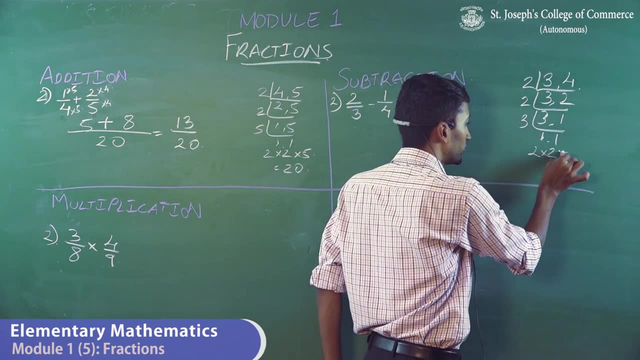 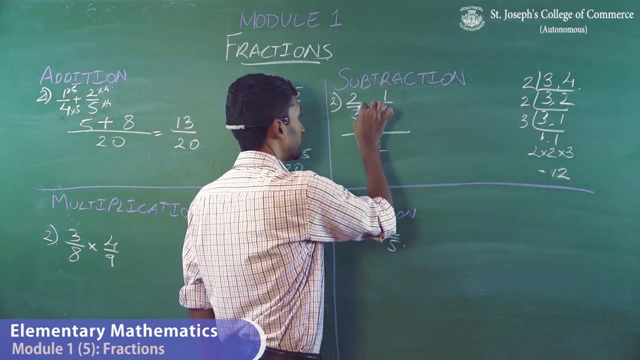 So 2, 2s are 4,, 2 1s are 2, and 3: 1s are. So 2 into 2, into 3 will give you 12.. So if 12 is your denominator, 3, 4s are 3.. 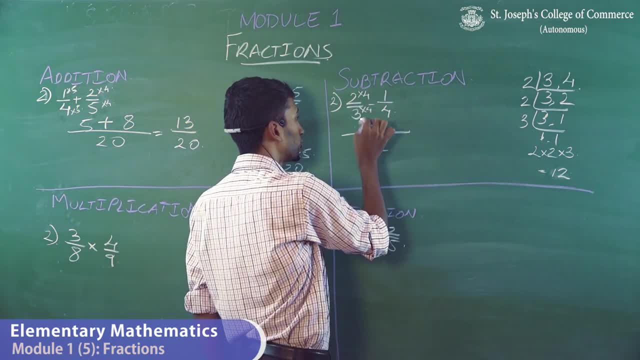 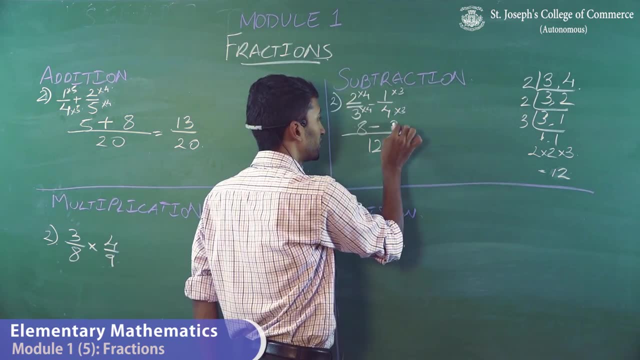 4s are 12, so you multiply the numerator also by 4.. 4- 2s are 8.. Minus 4, 3s are 12, so you multiply the numerator also by 3, that will be 3.. 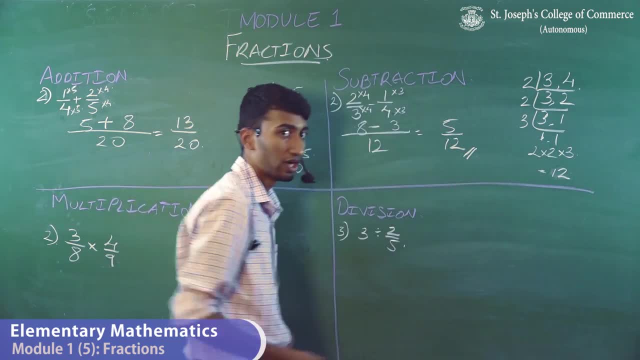 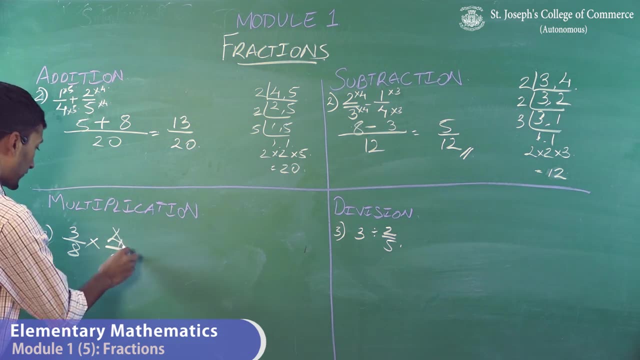 So 8 minus 3,, 5 by 12.. This is your answer. So we now move into multiplication where, since there's a multiplication sign, you can cancel out the common factors: 4: 1s are, 4, 2s are, 3, 1s are and 3, 3s are 9.. 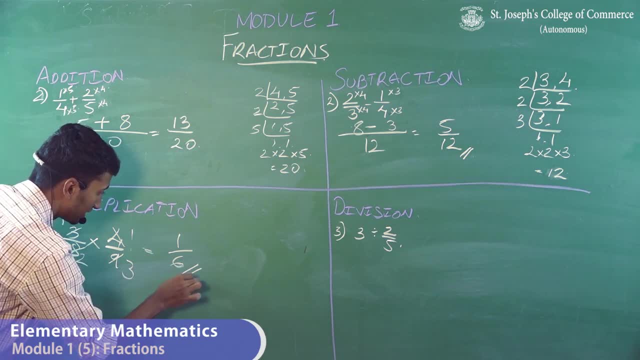 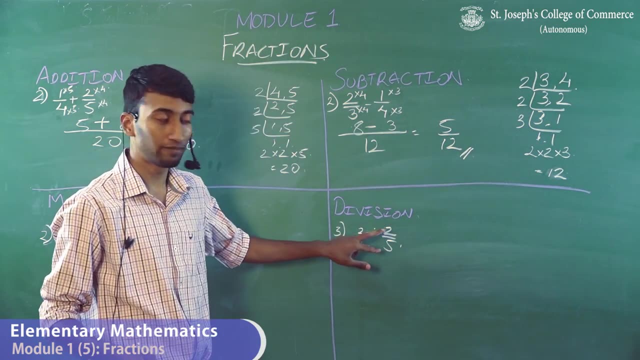 So 1 into 1 will give you 1,, 2 into 3 will give you 6.. So 1 by 6 is your answer. Moving into division, since there's a division sign, you have to reciprocate the second part. 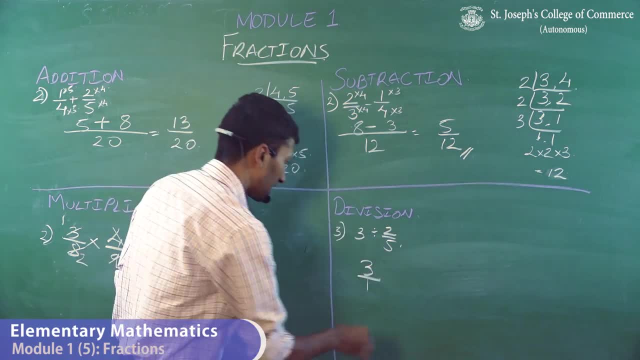 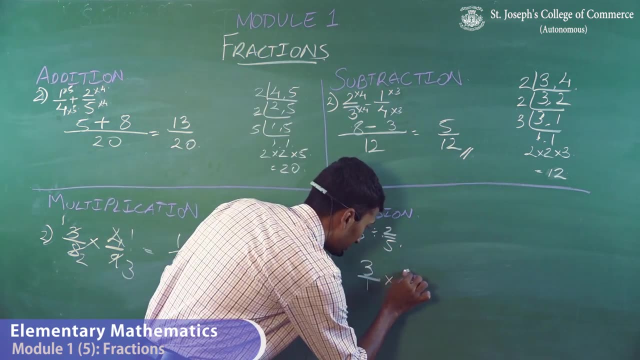 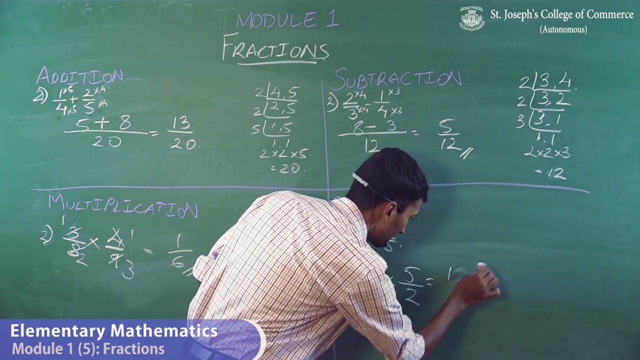 So that means I can write 3 as 3 by 1, multiplication sign, and then after that you reciprocate the other fraction, That becomes 5 by 2.. So 5, 3s are 15, and 2, 2, 1s are 2.. 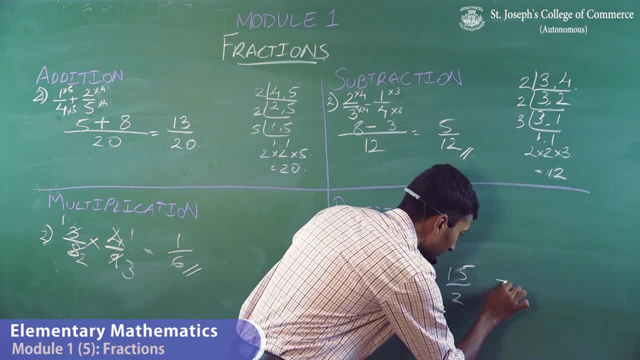 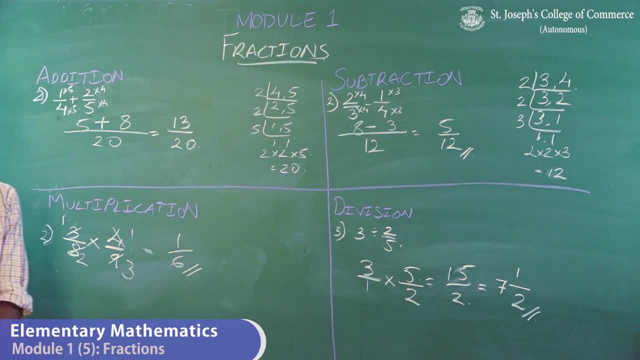 And you can't leave it in an improper fraction, so you have to convert it. 2, 7s are 14, 1 is a remainder by 2.. So 7 and a half is your answer.